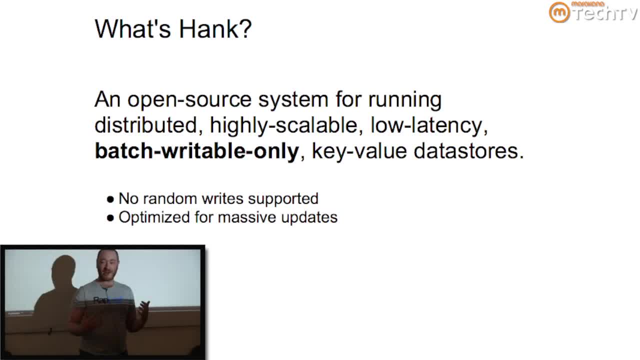 do crazy stuff to make it really fast and optimize very, very heavily for these massive writes. So it's not like 10 writes, it's like 100 million writes And that's what we're built for And key value. So this is a NoSQL project, if you guys are familiar with that. 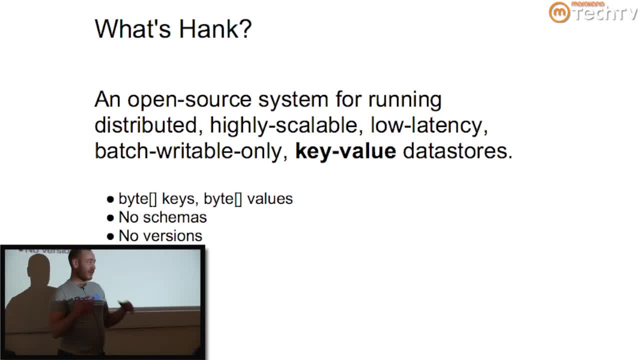 term Keys are byte arrays or values are byte arrays. There's no schema at all And there's no versioning or other stuff. you might see with more complicated NoSQL projects And, more specifically, we took the approach of making this just as simple as possible to fill this. 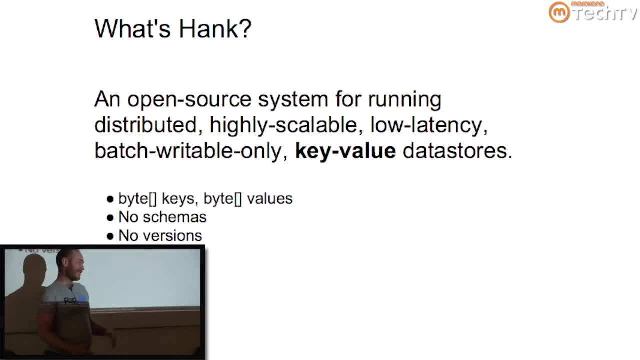 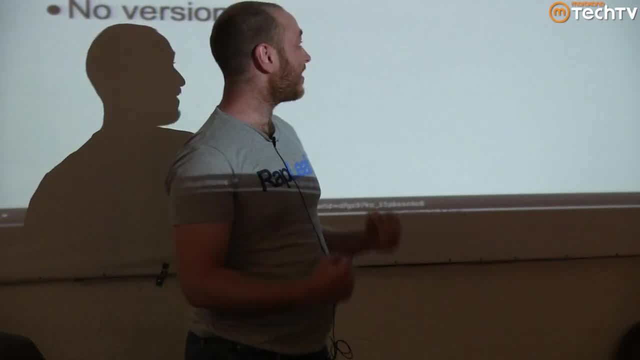 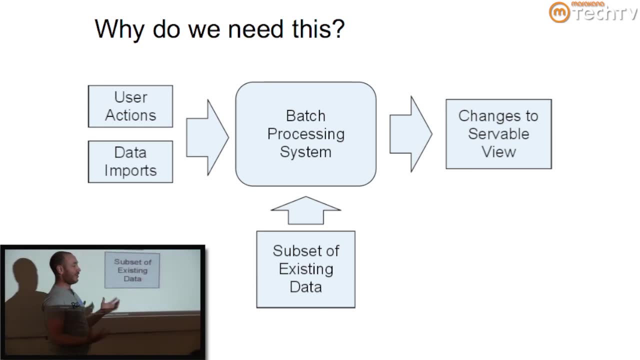 basic workflow, so that we didn't have to worry about supporting crazy consistency guarantees or weird versioning systems or timestamps or anything else. It's just fast, simple, key value. So why do we need this? Okay, so this is an extremely simplified view of what our system 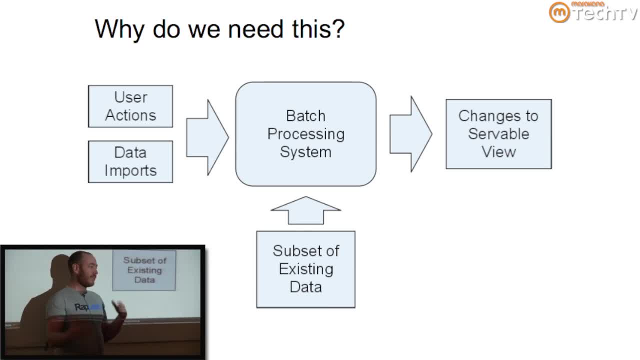 looks like We have user actions and data imports that come in synchronously or asynchronously and they get batch processed together with just a subset of the data we already have stored from all of history. okay, And so we've made it. so it's efficient for us to take just 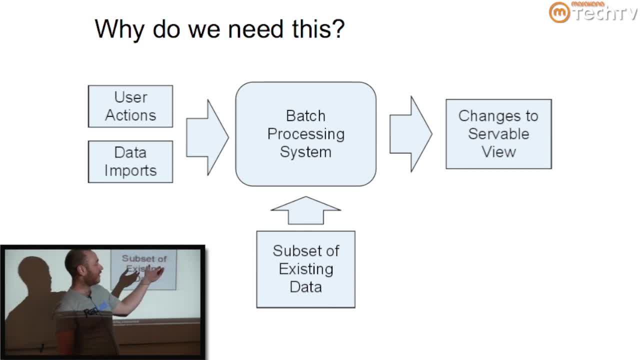 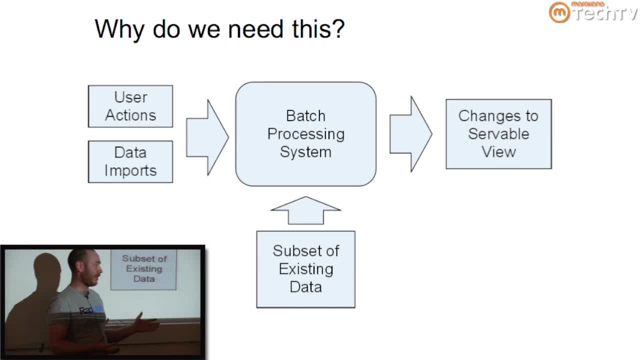 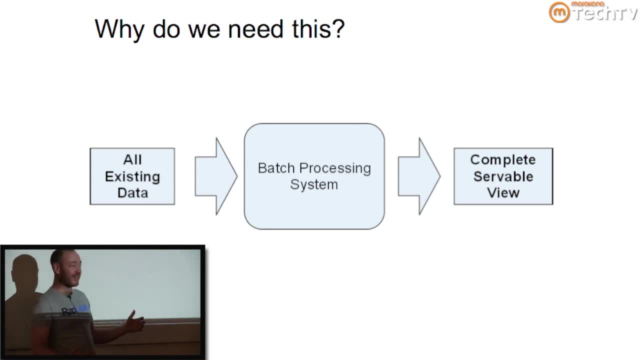 It's not imm véritable in the MySQL or traditional techniques, and that's completely true, And you can scale MySQL. I wouldn't want to say that's not possible. But what's really challenging is this: Once in a while, instead of doing just a little data, we do all of. 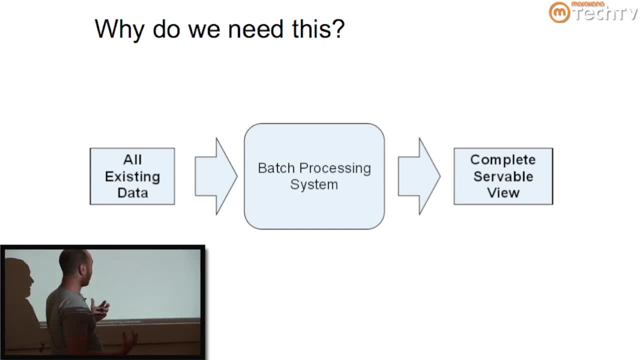 it. Whenever we change the way that we analyze our gigantic datastore, we throw all of our output hours out and start over from scratch. okay, And no datastore we could find could handle the volume of just being completely refreshed once a month or every two months. or so. So we built something that makes this possible. Lastly, we've taken a few more common problems happen if we try and dress that up and sort a process for the data and see if they're loggenly compatible, and things go wrong. so we as basically 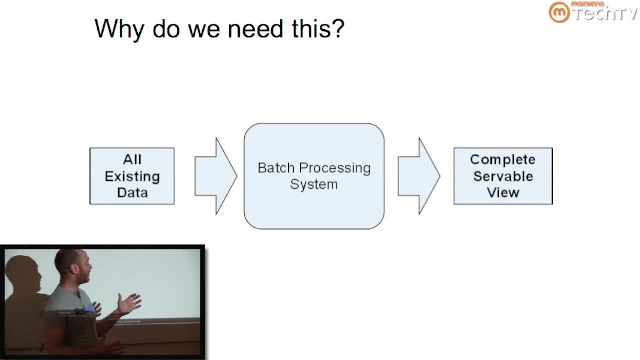 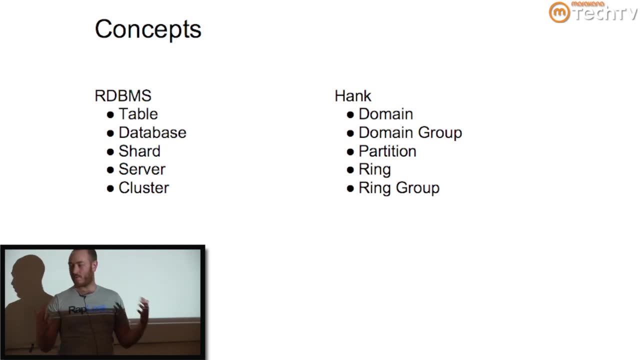 possible. Let's quickly talk about some concepts. I think everyone here is pretty comfortable with the whole relational database, slash MySQL kind of world. Let's compare that to what Hank does In a database. you have a table In Hank. we call that a domain. There's just. 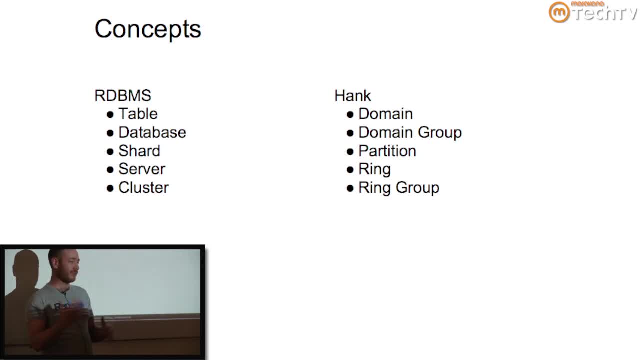 little differences. Basically, a table has columns and rows. In Hank you just have keys and values. It's just a simplified map. It's like a hash in Ruby, Again very elemental In a relational database. you have databases which are collections of tables. We have that. 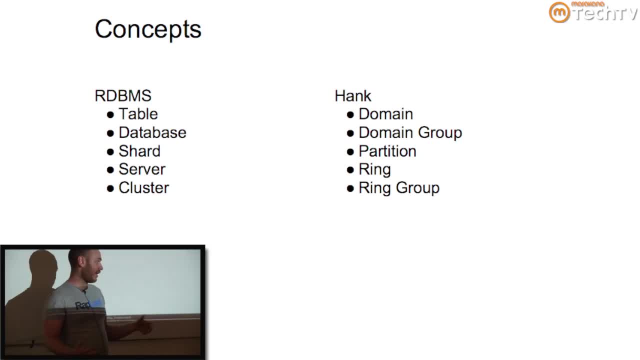 same kind of concept in Hank and it's just called the domain group. It's just an arbitrarily wrapping of domains into groups that you're going to use together for a particular application. Now, when you get to scaling relational databases, you might have shards, which is where you 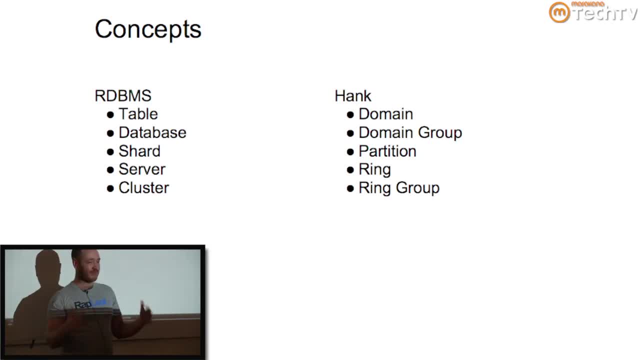 put the parts of the table on different actual physical database machines to get more throughput or capacity or whatever. We have something very much like that which is called a partition. Partition and shard are pretty much interchangeable In the Hank terminology. it's partition. It's really important for us to be able to grow. 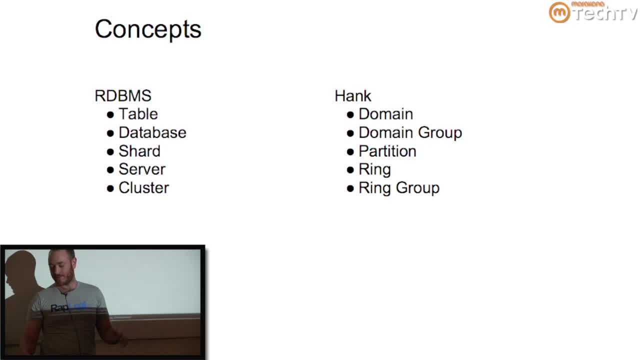 and spread the partitions over bigger and bigger groups of servers as we get bigger In a relational database. you have a server In Hank. we don't really have just one server. We have this thing called the ring, which is like a collection of servers that together 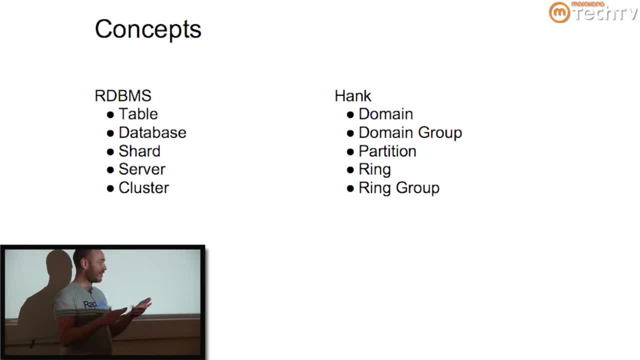 can give you a complete view of all the data. It's really clear from the ground up that this is about many servers working together to accomplish your overall data serving goal. Then, instead of a cluster, we have this thing called a ring group, which is obviously a. 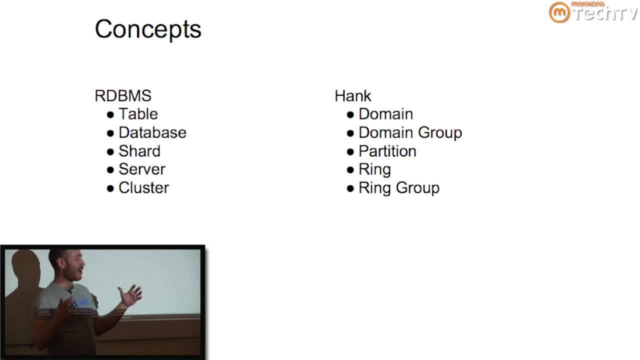 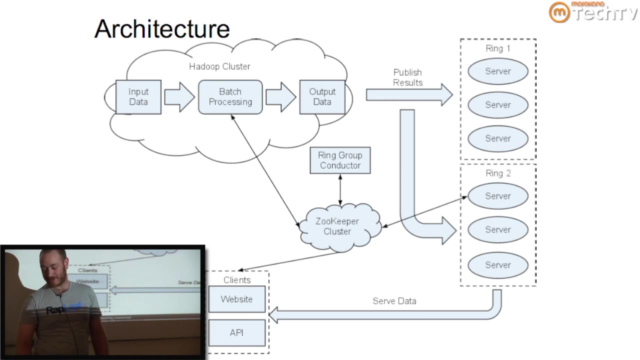 group of rings. There's this nice hierarchy of data and deployment that makes it work well together. A lot of the same concepts, just with different names and slightly different functionality. Here's that same thing, but drawn in a nice diagram which I'll talk through. 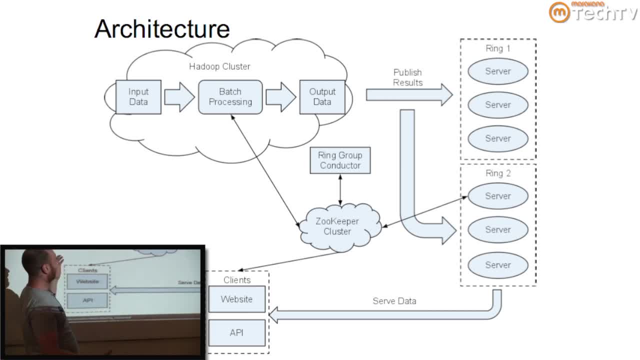 quickly. This roughly reflects our workflow and how things happen. We have all of our input data and our existing data stored in a giant database. We have all of our input data and our existing data stored in a giant database. It's a gigantic Hadoop cluster. As of last count, it's about one and a quarter petabytes. 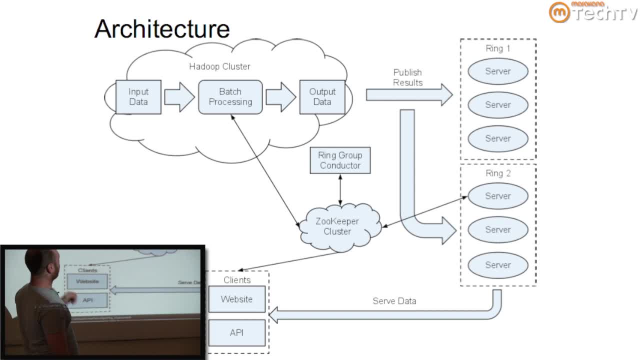 of storage and we fill it like 80%. It's pretty exciting. We do our batch processing and we get this raw output data. that's organized really well for serving, but now it's on 400 machines. It's not really convenient for us to put it on our website. We have this process. 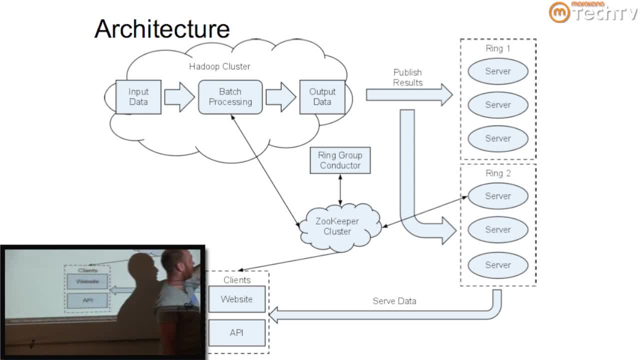 whereby we take this output data and we publish it to servers close to our front-end which are optimized for serving really, really fast, small values. This is where the random access happens, okay, And so the publishing it's coordinated by this thing we call the ring group conductor. 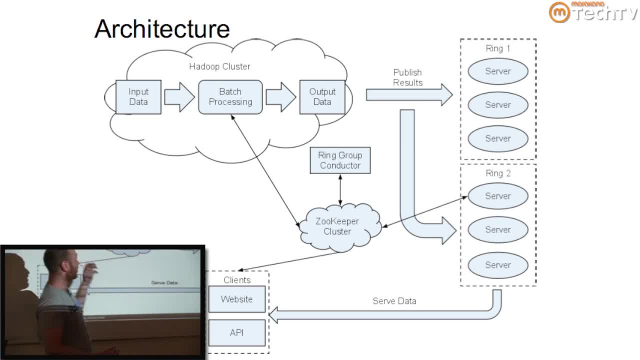 which is like a single daemon who watches for changes to domain groups as they happen and then, like, tells servers to come up and go down in sequence to get the data out- And something that's not obvious from this diagram, necessarily. but when a ring is updating, it's also not serving okay. 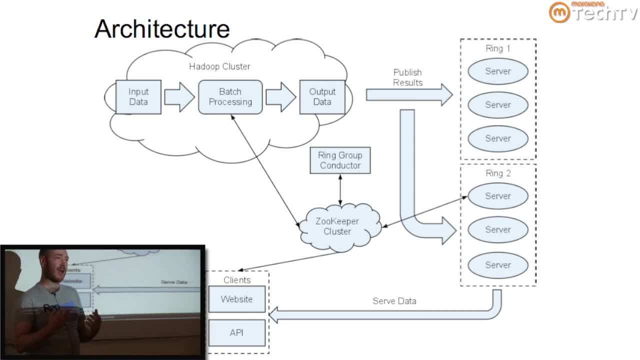 So it's really important for us that we had, like we always found that whenever you were updating while you were serving reads, the read performance of that shard tanks and that's no good Like if we see like a third of our requests are suddenly taking ten times as long. 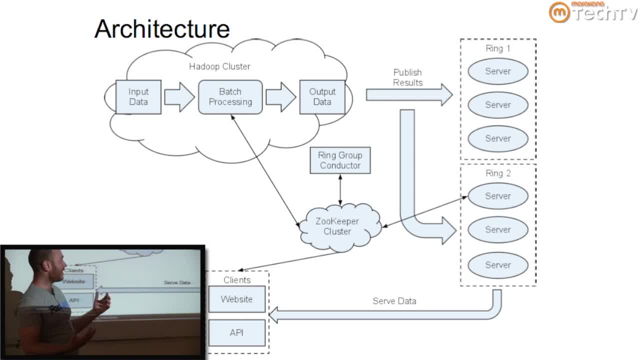 our customers are going to notice and we just can't bear that right. So this system, basically it isolates the writes and reads completely, Like you'll never see a read on a server that's writing and vice versa. So then, once the data is pushed out to these servers, 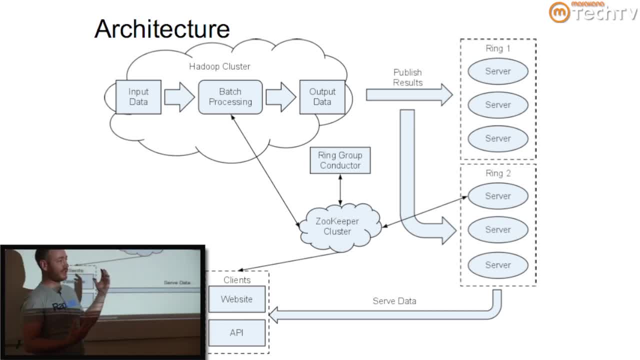 we use ZooKeeper, which is an Apache project for configuration management and locking and presence and stuff like that. Really cool project. It like maps partitions to servers for us so that the client down here- whether it's like the website or an API or any kind of client you might imagine- 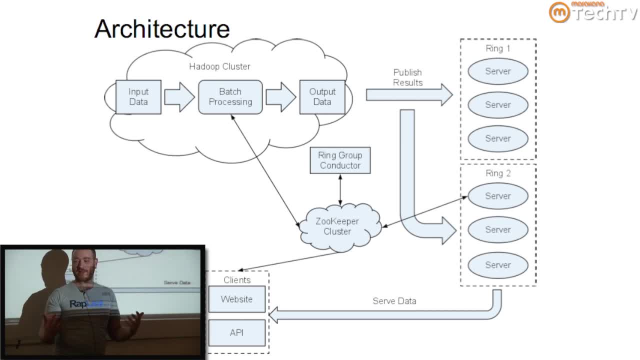 can figure out. okay, well, I have this key, Where do I go to fulfill? where do I get the value for that? okay, And it gets an address, goes and gets it and pulls the data through. So we've got this really nice blocked-out system so that like: 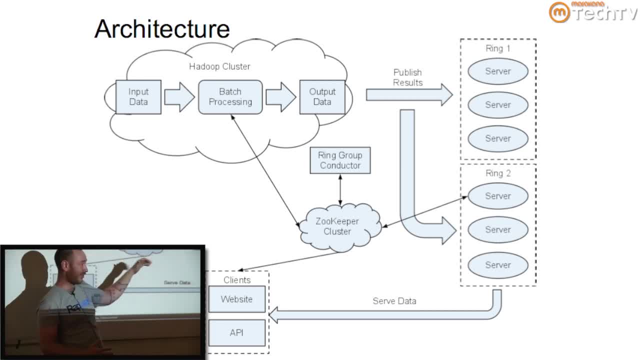 everything is in place. Everything is very predictable, Like. the cluster can go down and it's not a problem. The servers can go down and the cluster can still write data. Some of our servers can go down in the rings and the clients can still get it from other ones. 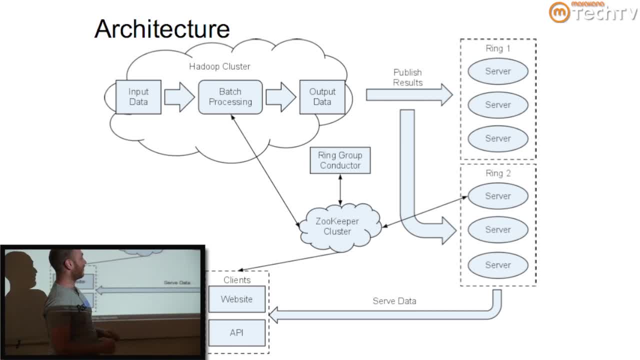 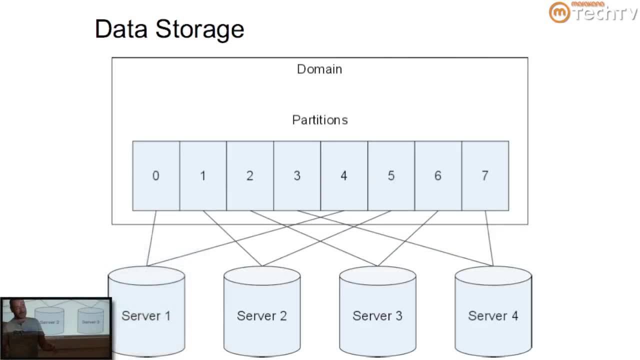 So we have great redundancy, We have great scalability. It's a pretty awesome system. But I tried to toot my own horn there, but it's really exciting. So to get a little deeper into, kind of what this looks like, so I mentioned partitions, right? 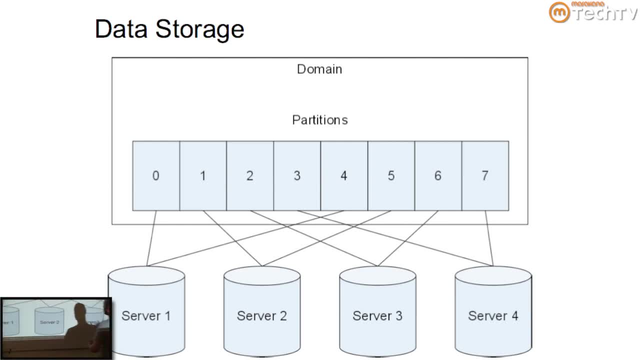 So we have a domain and it's broken up into kind of just arbitrary groupings- right, In this case there's eight partitions, but in practice we use more like 1,000, right, Basically, imagine how big you might want to one day scale it to okay. 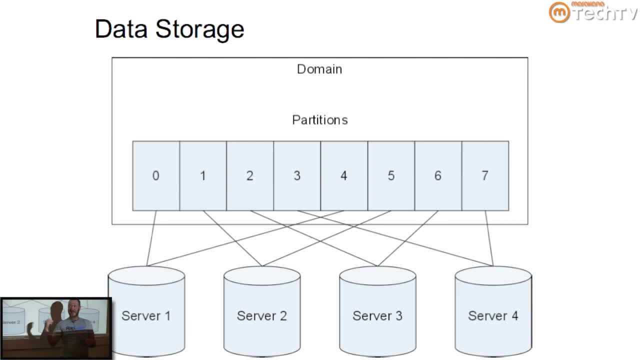 And those partitions are assigned to servers in like a static mapping. It's not just like a random hash mod thing, It's literally whatever you want it to be. So you can make really cool strategies for putting partitions on servers and get really nifty results as outcome. 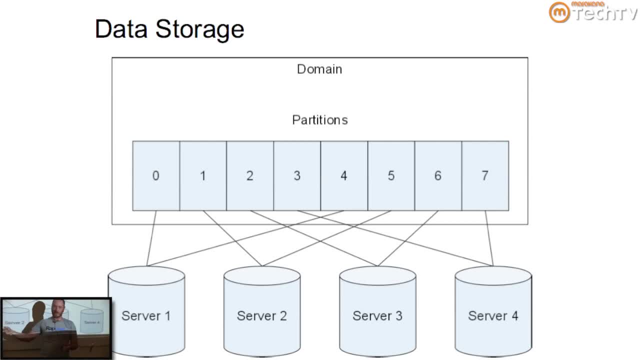 And you can see kind of from the lines here, you can actually assign a partition to more than one server, so you have redundancy kind of built in And that's beyond rings Like. you can also scale your capacity by putting every partition. 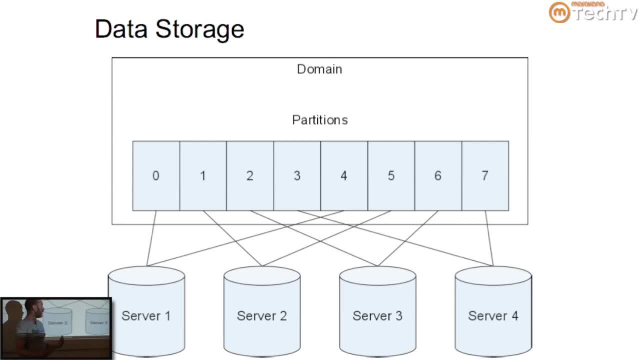 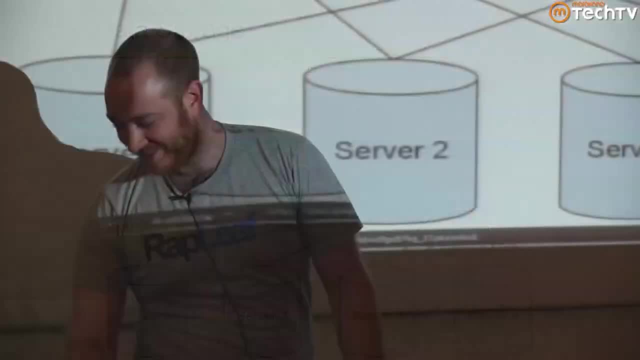 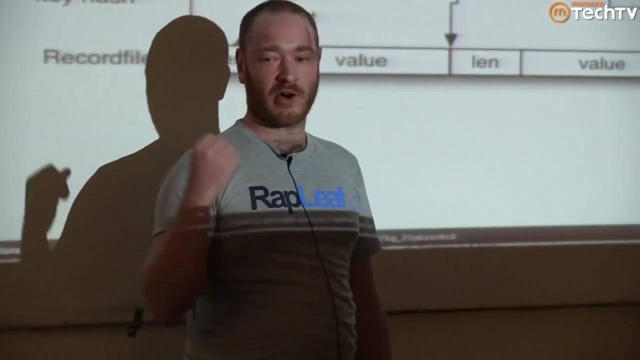 I mean every server, if you had to, But fundamentally it's just a very, very, very flexible system for scaling and scaling- Sorry. And then just one deeper thing to look at. Like I said, it's really important for us that our requests are like a millisecond. 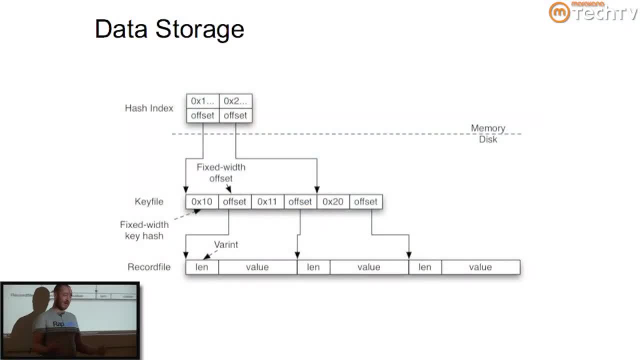 To make that happen, we had to work hard, Like a lot of people will say like: oh, try BDB or try this flat file or that, Don't do that, It's not any good. okay, It doesn't work out in the long run. 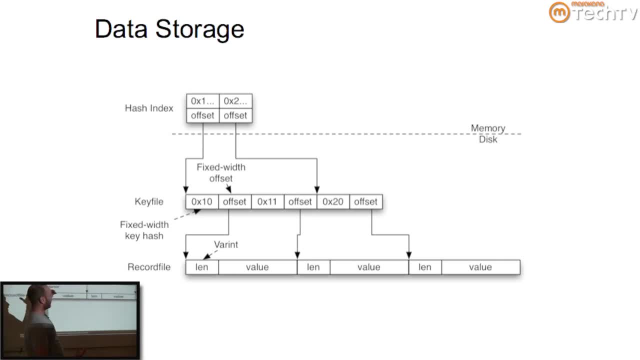 Okay, We had to build our own thing, which basically is a very careful kind of stack of some part in memory that helps us get to where we have to go really fast, and then exactly two places on disk that we can get to with like a minimal number of seeks and get exactly what we want. 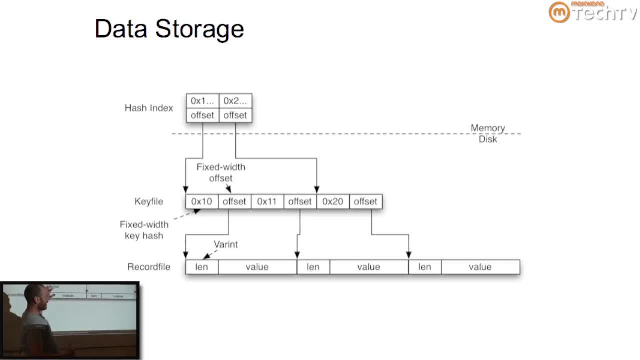 And like even further. like I could go into this in depth, but it's probably not that interesting. But the cool part is that even though this is really fast- like you never do more than two- seeks to get a value. 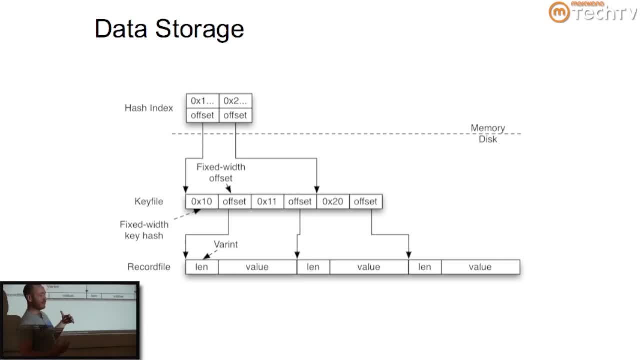 which is really quick. it's also really amenable to being merged, like big deltas that come in, Because it's basically just a big sorted flat file and you just zip it together like merge sort with small deltas as they come out of the Hadoop cluster. 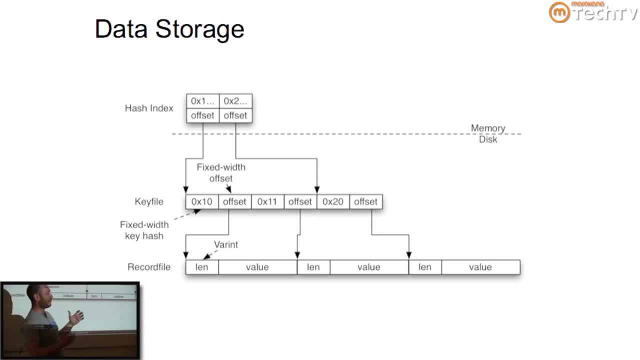 Okay. So basically we get this good mix of really fast random access performance and really fast batch merging performance when you put it all together. So this is what we're really proud of. This is a really cool system and it gives us great performance. 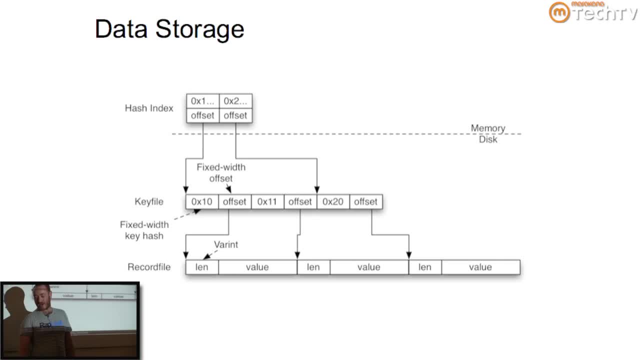 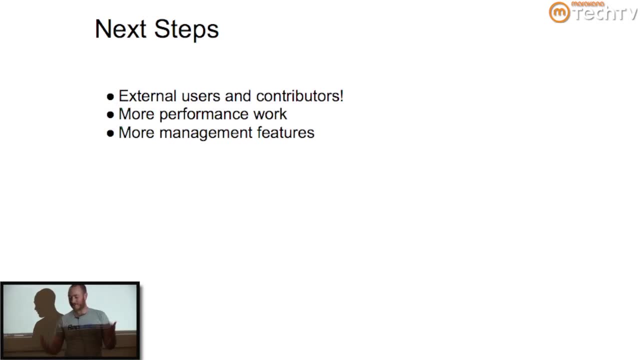 and it backs our APIs and website and everything. So the next steps for the Hank project: like I said, I'm talking to you guys today because we're trying to get the word out there about how cool this is. We'd love, would love- external users and contributors.